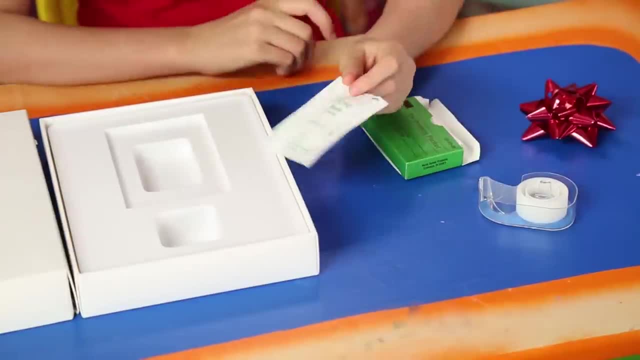 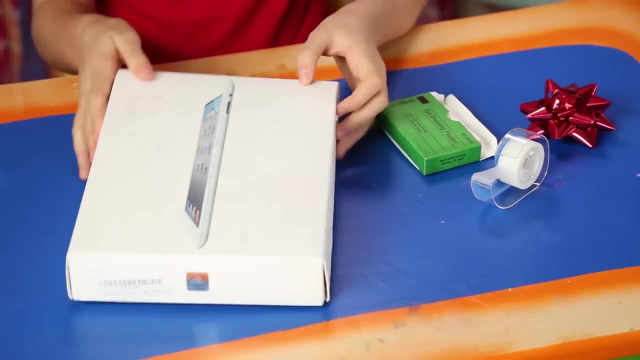 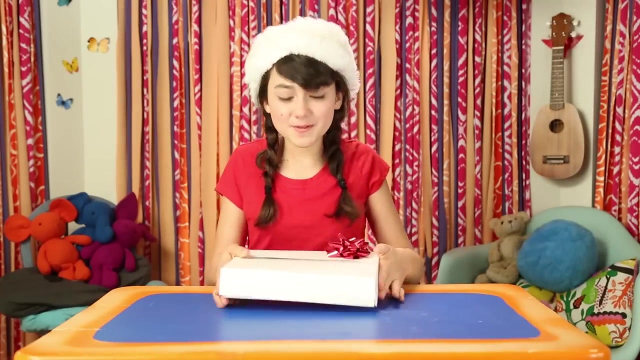 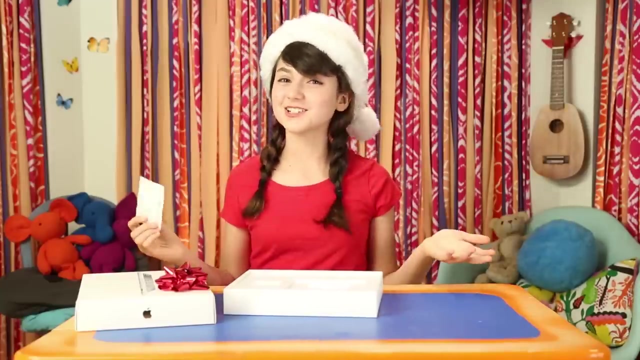 Open the iPad box, Tape the iPad gauze inside, Close the box, put on the bow and you're all set. I can't believe you got me an iPad- The Not-So-Rad iPad- Guaranteed to bring tears of joy and laughter. 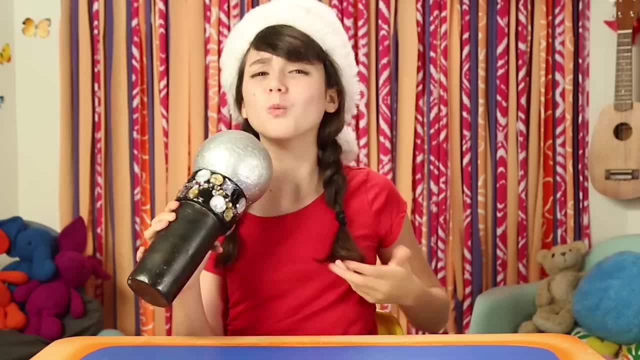 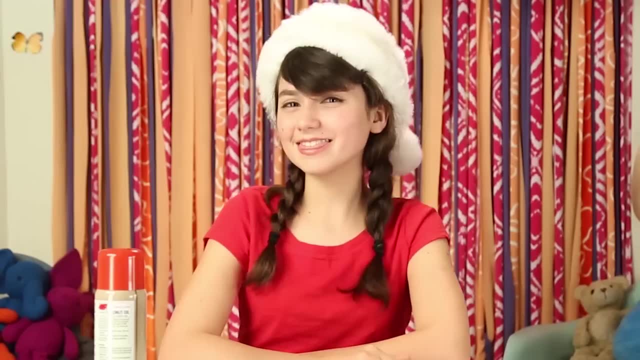 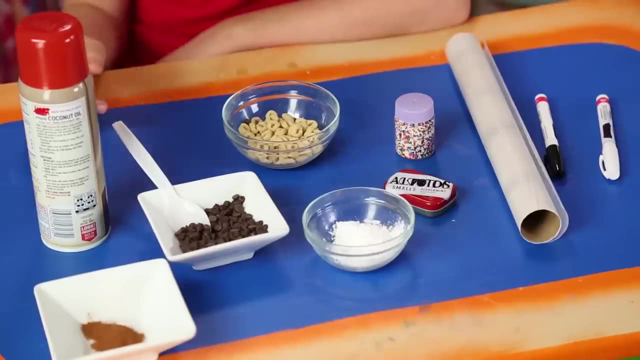 Speaking of laughter, here's a quick joke for you. What kind of deer helps the grass grow? A reindeer. Let's get some yummy in your tummy with an elf-sized snack: My dinky donuts. For this you'll need cooking spray, cinnamon, chocolate chips, a spoon powdered sugar, Cheerios, a mint, tin sprinkles, white and black paint, markers and waxed paper. 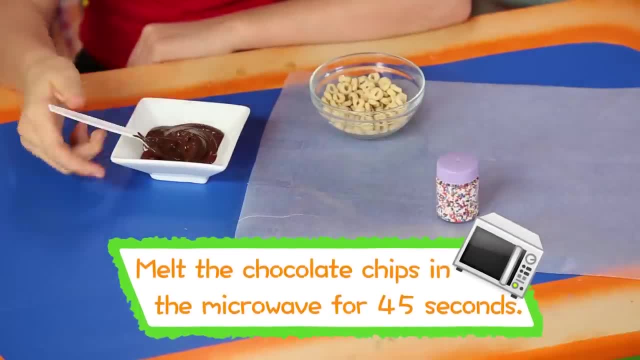 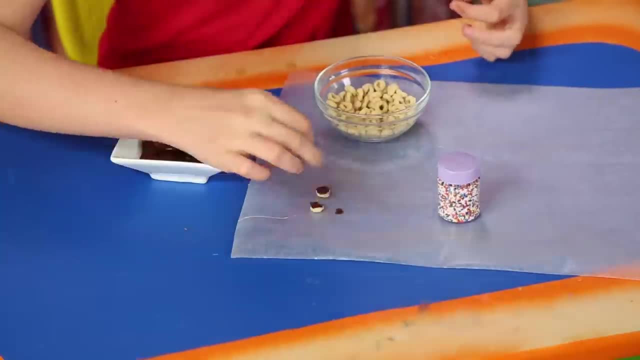 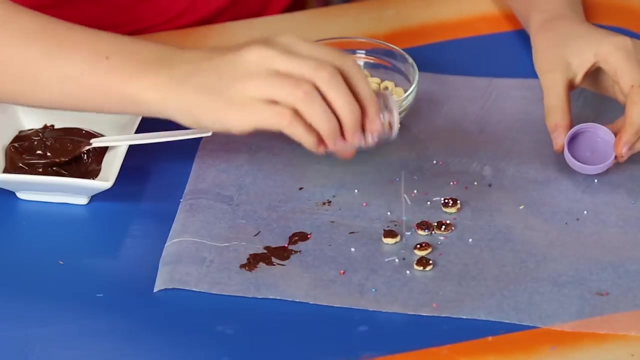 Melt the chocolate chips in a microwave for about 45 seconds. Dip one side of a Cheerio into the chocolate. You can remove extra chocolate by dipping your Cheerios onto the wax paper. Then add sprinkles. Next, spray a few Cheerios with coconut oil. 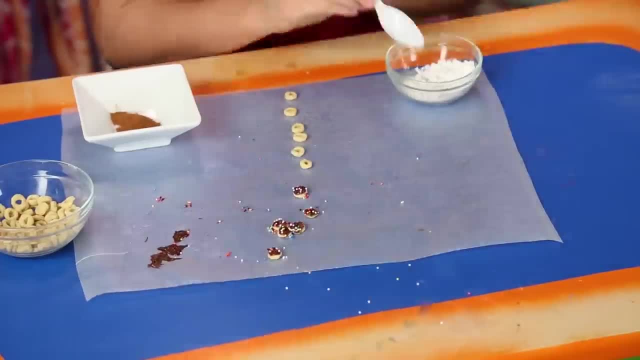 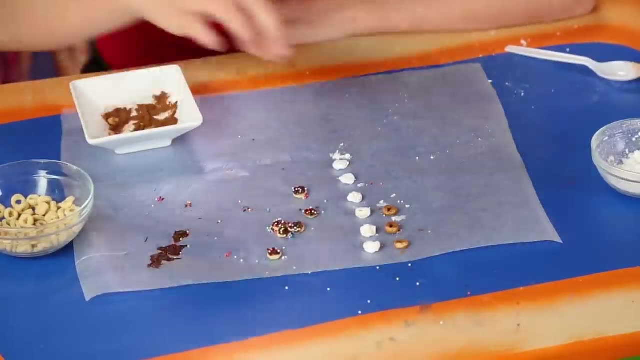 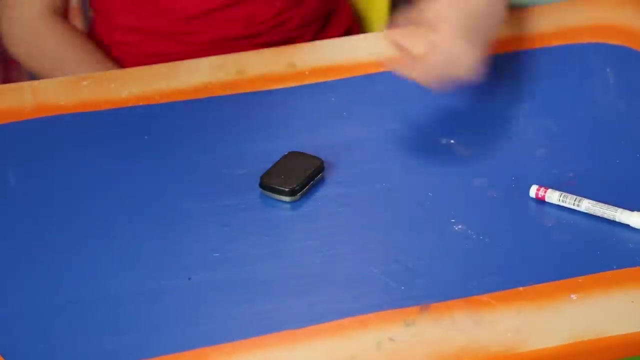 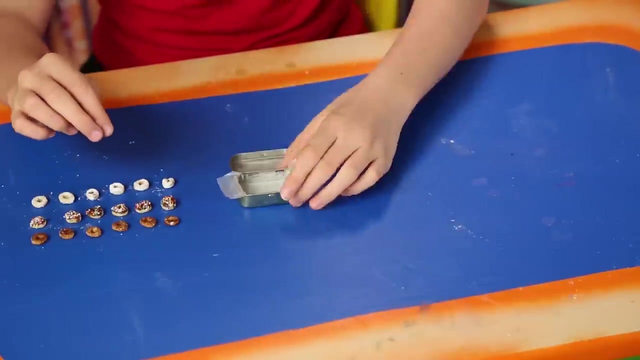 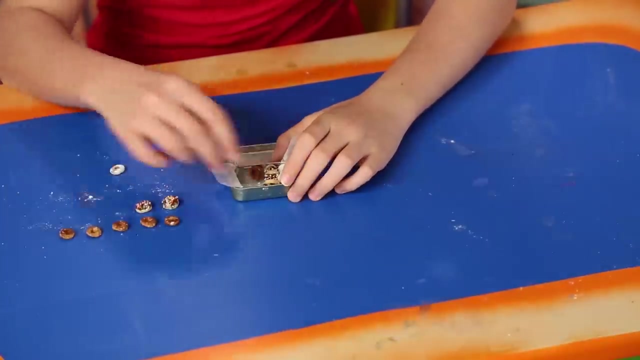 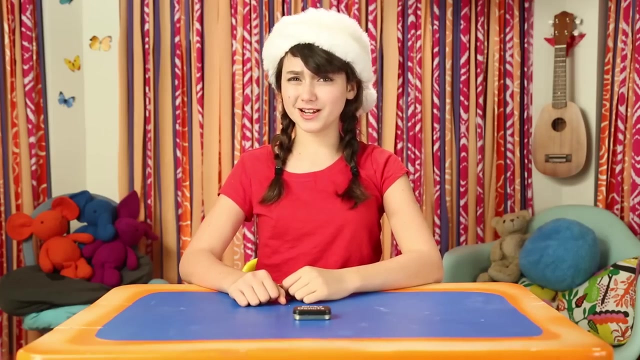 Dip some of them in the powdered sugar, Then dip the rest in the cinnamon. Decorate the mint tin And line it with wax paper. This will be your dinky donut box. Place your donuts inside, All done. Next time your friend says she's a little hungry, give her a little snack. 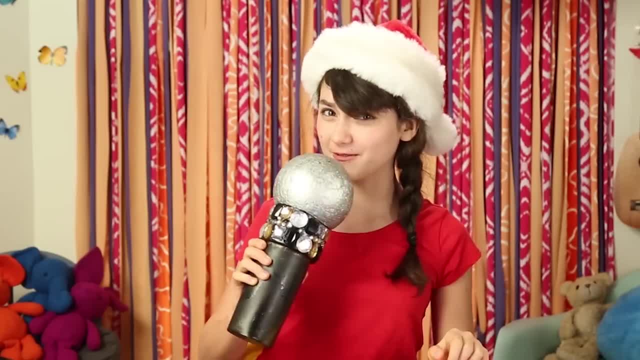 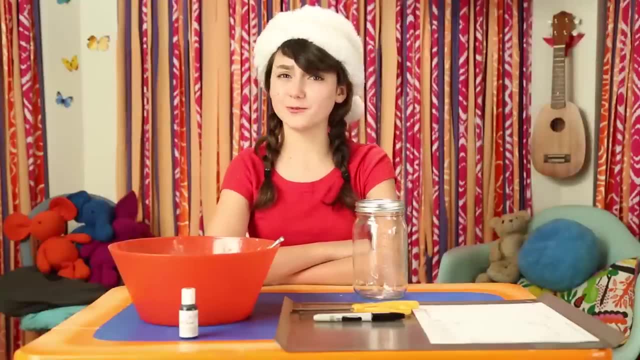 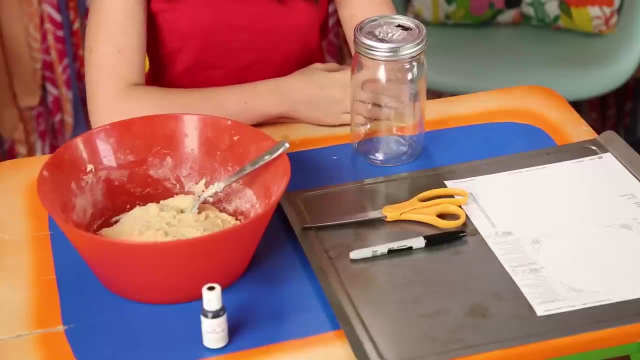 Quick joke number two: What's a bee's favorite holiday? Hanukkah. Even if your friend has been really naughty, this final hack tastes really nice: My big ol' lump of coal. For this you'll need a mason jar, label paper scissors, a black marker, black food coloring, baking sheet and sugar cookie dough.